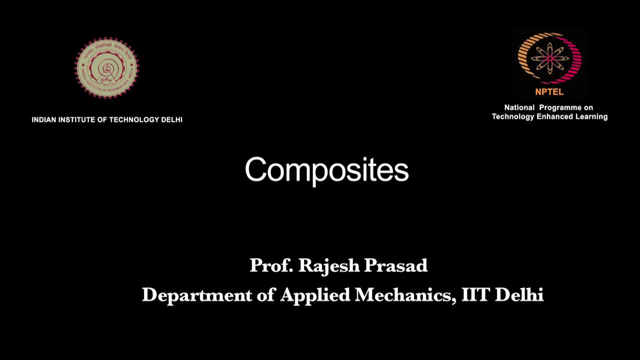 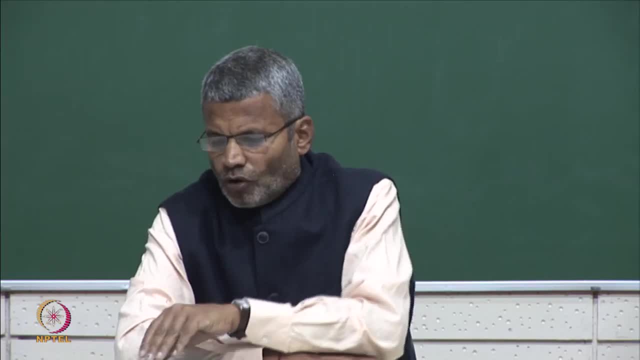 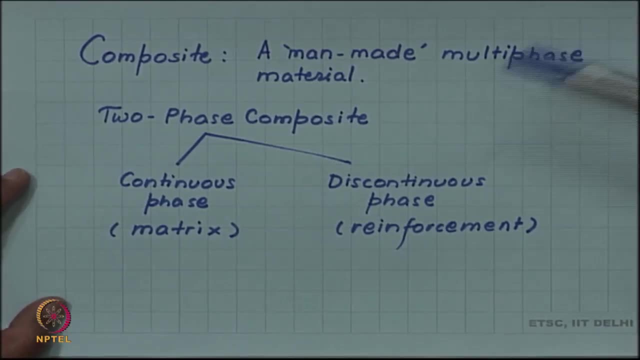 An important class of material is composite materials. By composite material we mean a manmade multiphase material. We have met multiphase material previously, like steel, in which ferrite and cementite is there, but that we will consider because ferrite and 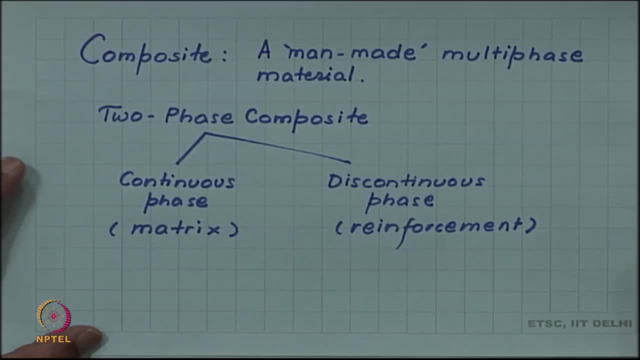 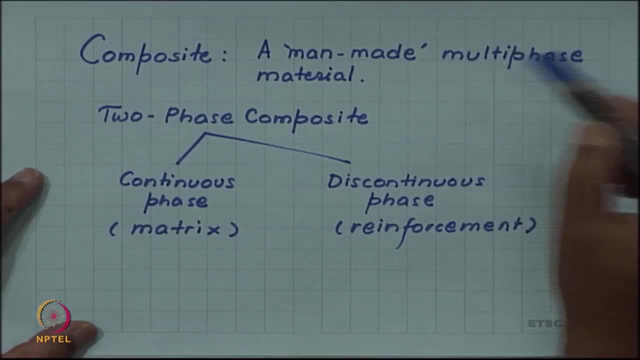 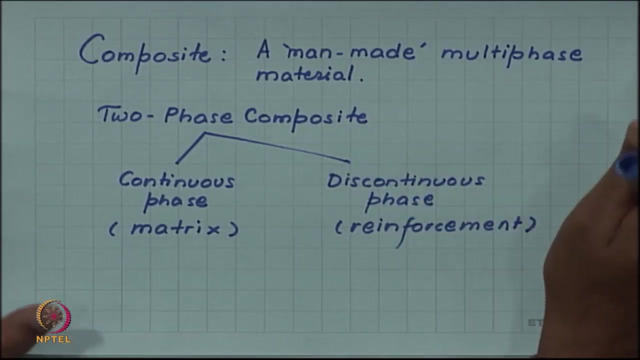 cementite. both phases form during natural cooling of a steel from the austenite phase, So that by manmade we mean that the two phases were individually existing and then they were put together to form this composite material. Out of two phases, one is generally a continuous. 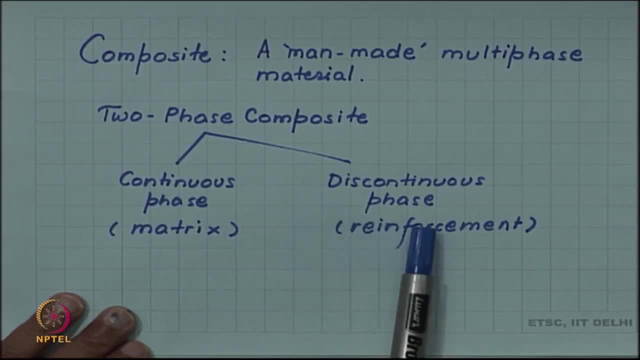 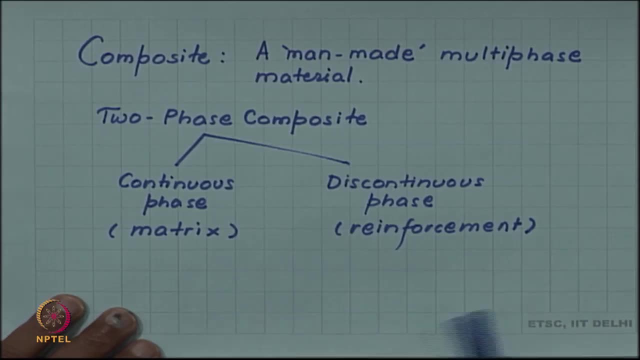 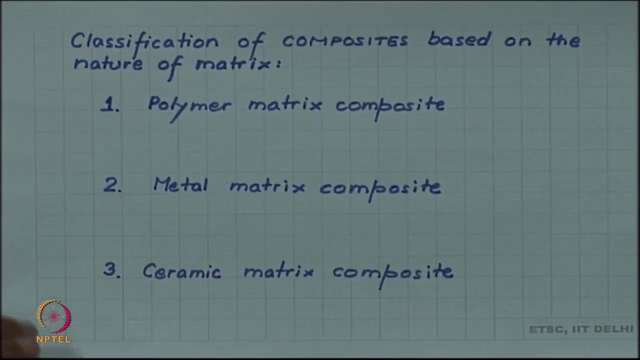 phase, which is called matrix, and another is discontinuous phase, which is called reinforcement, Although in some composites, like sandwich composite, both phases may be discontinuous. Now composites can be classified on the basis of the nature of matrix. So we have polymer. 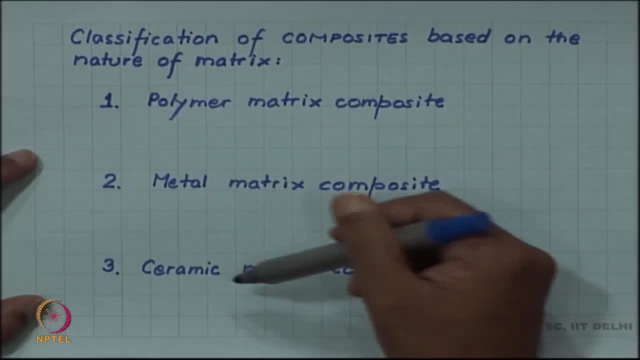 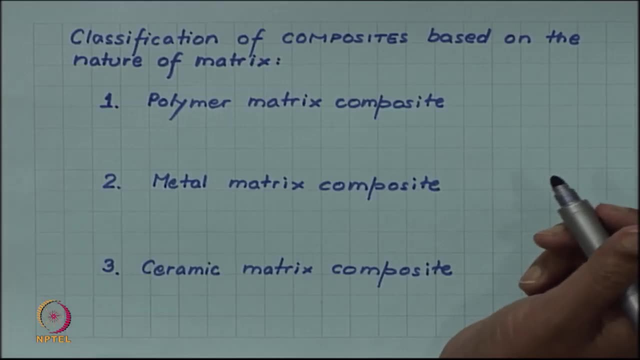 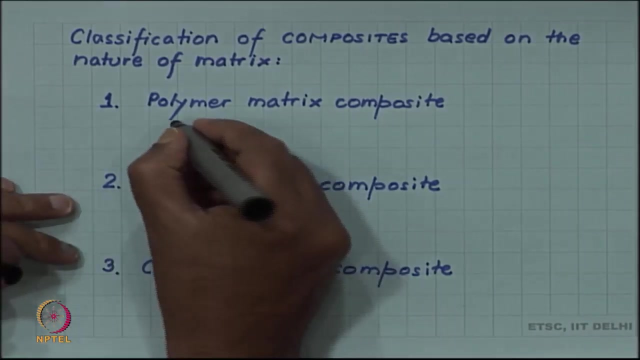 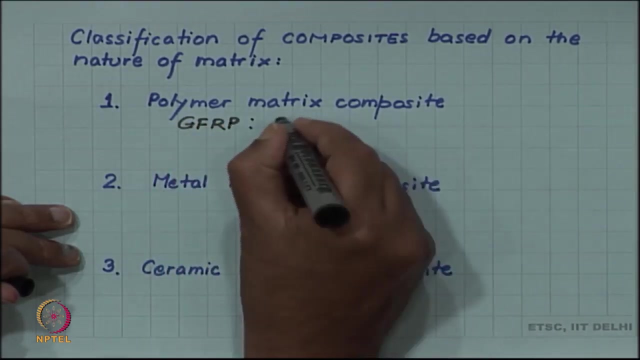 matrix composite, metal matrix composite and ceramic matrix composite, depending on whether the matrix is polymer or metal or ceramic. Example of polymer matrix composite will be, for example, GFRP, which is short for glass fiber reinforced plastic. glass fiber reinforced plastic. So GFRP is GFRP, So GFRP is GFRP. 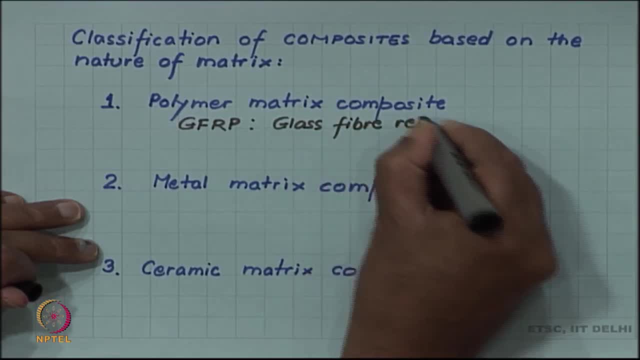 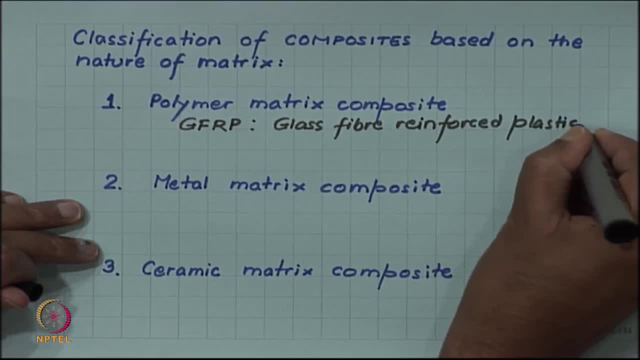 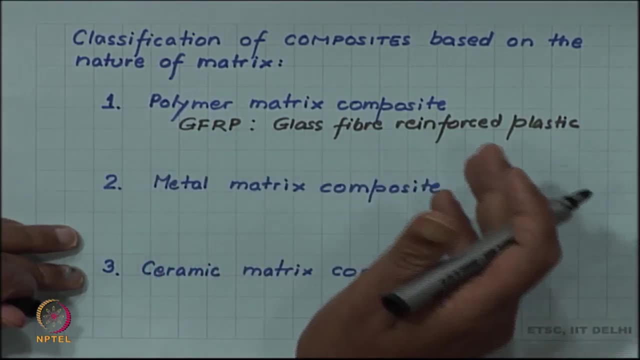 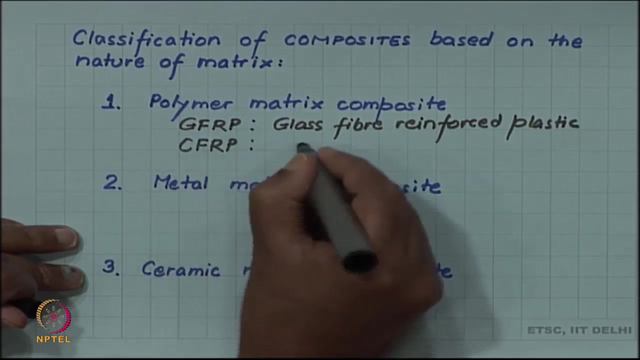 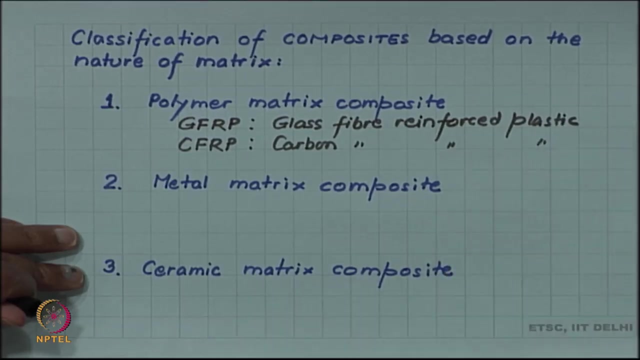 Reinforced plastic, Reinforced plastic. so in this, in a plastic, for example polypropylene or epoxy, glass fibers are put. so that is glass, and for reinforcement So glass fiber, reinforced plastic. or we have CFRP, carbon fiber, reinforced plastic. Many times in a sports equipment.